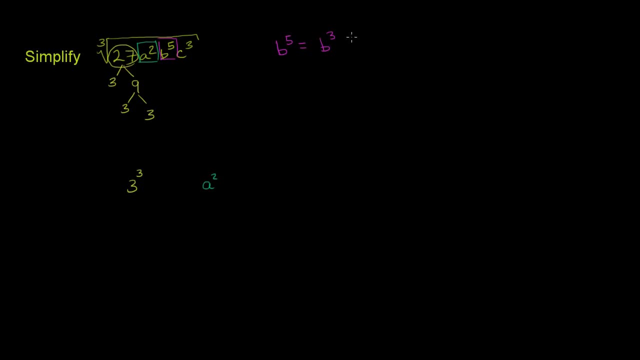 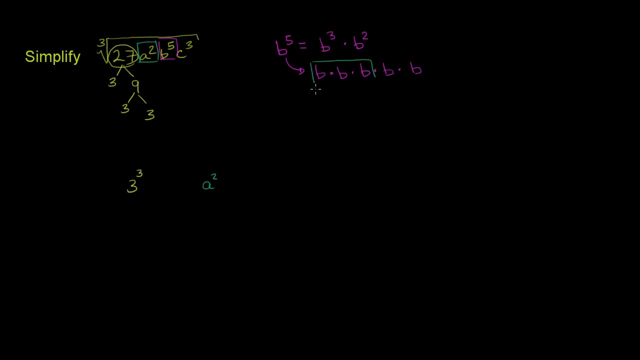 So this, the first three are clearly b to the third power, and then you have b to the second power after it, So we can rewrite b to the fifth as a product of a perfect cube. So I'll write b to the third. I'm doing that same purple color. 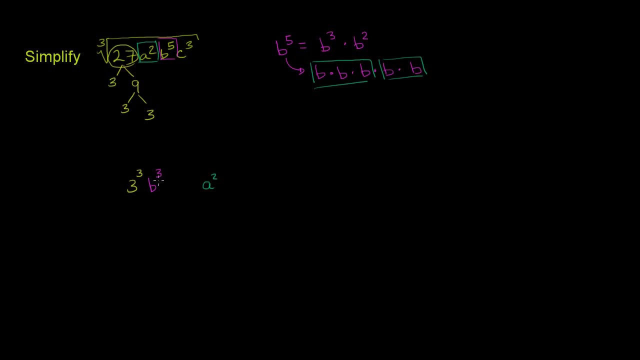 So we have b to the third power over here And then it's b to the third times b to the third power. So I'll write the b squared over here and we're assuming that we're going to multiply all of this stuff. 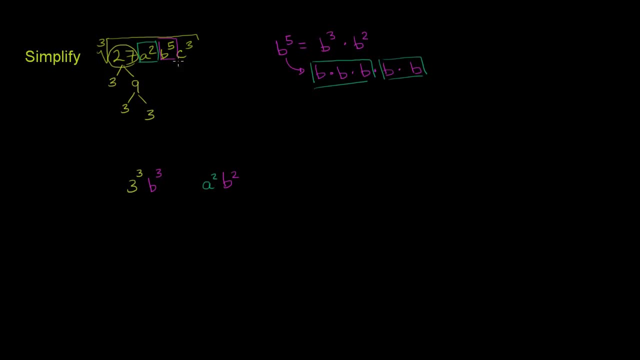 And then finally, finally, we have- I'll do it in blue- c to the third power. Clearly, this is a perfect cube. it is c cubed, it is c to the third power. So I'll put it over here. so this is c to the third power. 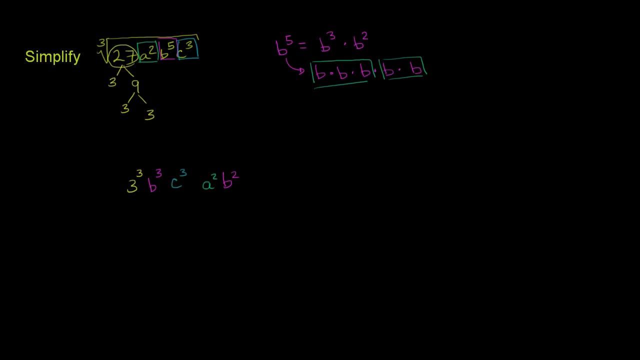 And of course, we still have that overarching radical sign. So we're still trying to take the cube root of all of this And we know from our exponent properties, or we could say from our radicals, radical properties- that this is the exact same thing. 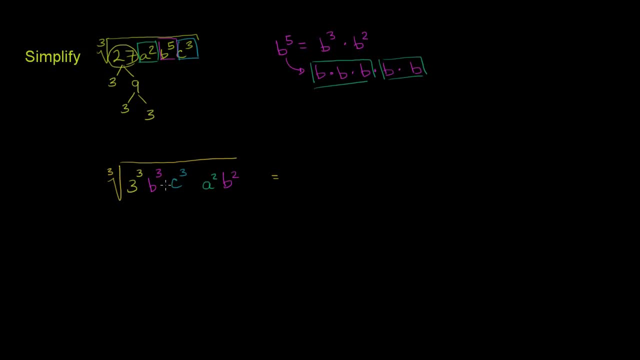 That taking the cube root of all of these things is the same as taking the cube root of these individual factors and then multiplying them. So this is the same thing as the cube root, and I could separate them out individually, or I could say the cube root of 3 to the third, b to the third, c to the third. 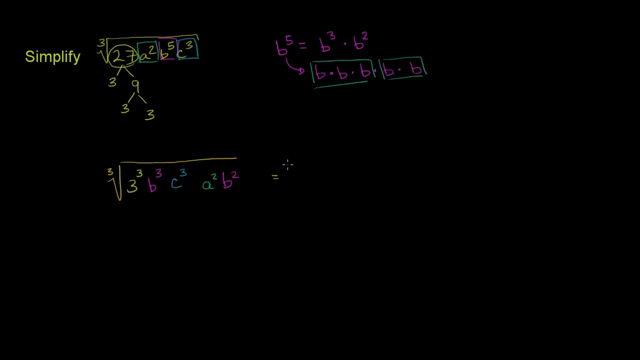 Actually, let's do it both ways. So I'll take them out separately. So this is the same thing as the cube root of 3 to the third times the cube root. I'll write them all in. well, I'll write it, do it. 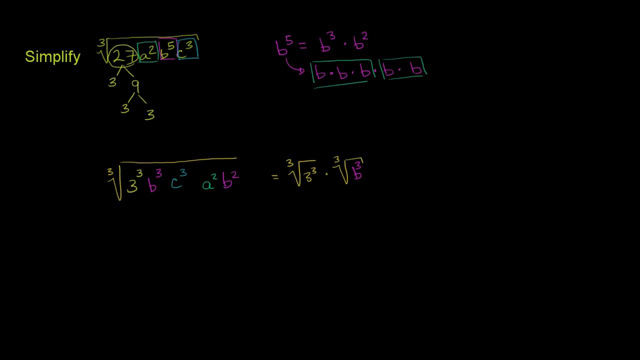 or code it so we don't get confused. Times: the cube root of b to the third times the cube root of c to the third times the cube root, and I'll just group these two guys together, just because we're not going to be able to simplify it anymore. 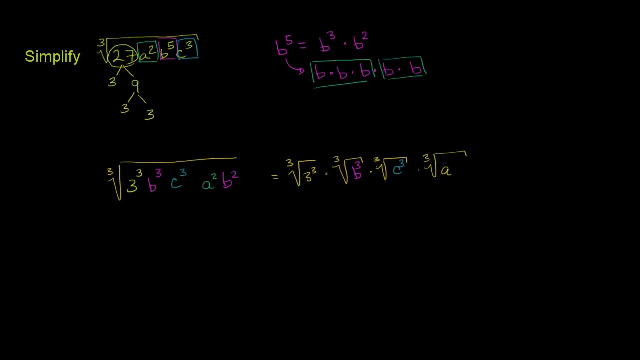 Times the cube root of a squared, b squared. I'll keep the colors consistent while we're trying to figure out what's what a squared, b squared, And I could have. I could have said that this is times the cube root of a squared, times the cube root of b. 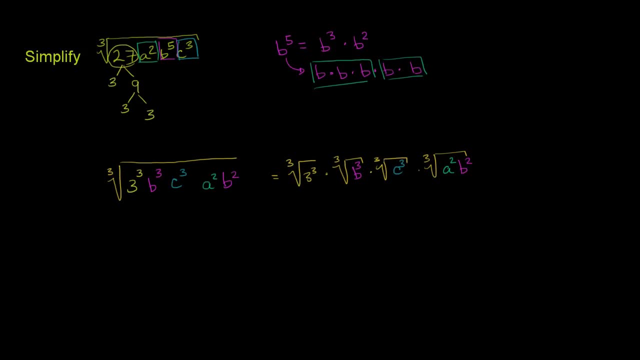 squared. but that won't simplify anything, So I'll just leave these like this, And so we can look at these individually: The cube root of 3 to the third, or the cube root of 27,. well, that's clearly just going. 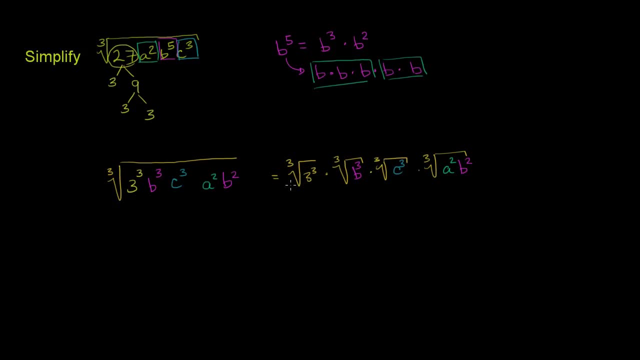 to be. I want to do that in that yellow color. This is clearly just going to be 3, right 3 to the third power. is 3 to the third power or it's equal to 27.. This term right over here, the cube root of b to the third. well, that's just b. 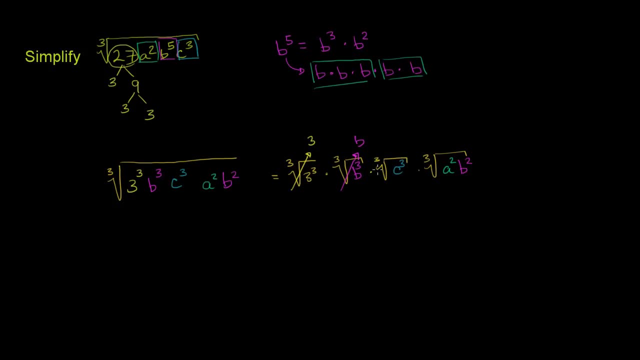 That's just b. And the cube root of c to the third, The cube root of c to the third. well, that is clearly just c. So our whole expression has simplified to 3 times, b times c times the cube root of a. 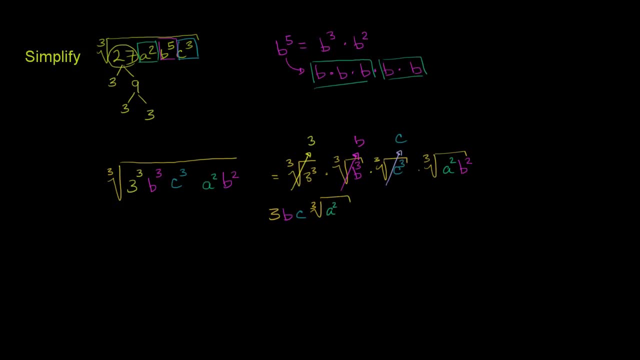 squared, b squared Times, the cube root of a squared, b squared, And we're done. I just want to do. I want to do one other thing, just because I did mention that I would do it. We could simplify it this way, or we could recognize that this expression right over 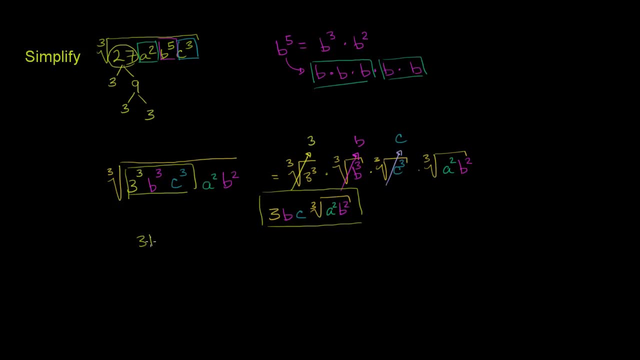 here can be written as 3bc to the third power. If I take three things to the third power and I'm multiplying it, that's the same thing as multiplying them first and then raising them to the third power Comes straight out of our exponent properties. 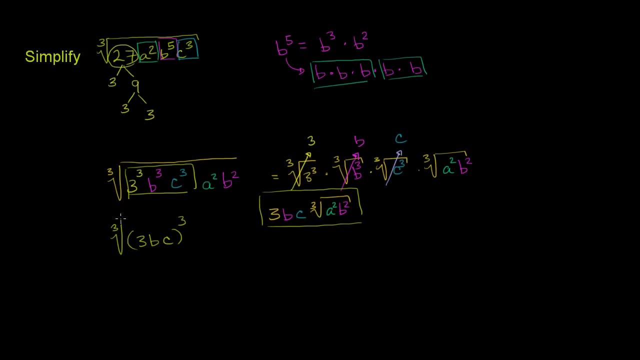 And so we can rewrite this as the cube root, the cube root of all of this times, the cube root of a squared, b squared, And so the cube root of all of this, of 3bc to the third power. well, that's just going. 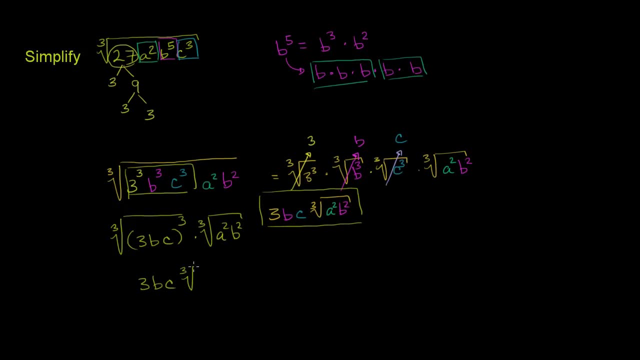 to be 3bc And then multiplied by the cube root of a squared, b squared. I didn't take the trouble to color code it this time because we already figured out one way to solve it, But hopefully that also makes sense. 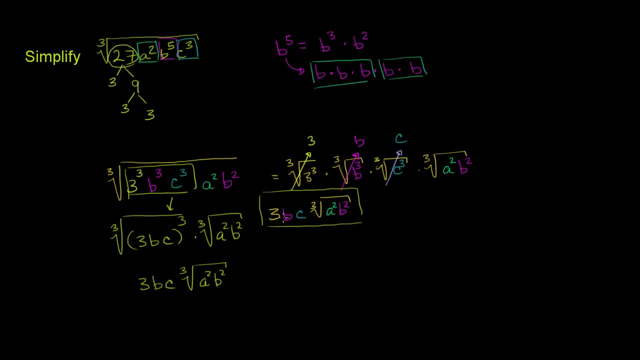 We could have done this either way, But the important thing is that we get that same answer.